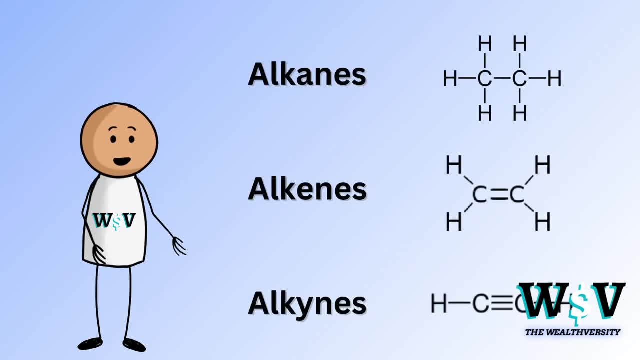 alkynes has only single bonds, while alkenes have double bonds and alkynes have triple bonds. If you would like to learn more about alkanes, check out our other YouTube video to learn more. So what is the general formula for alkenes? The general formula for alkenes is CnH2n. 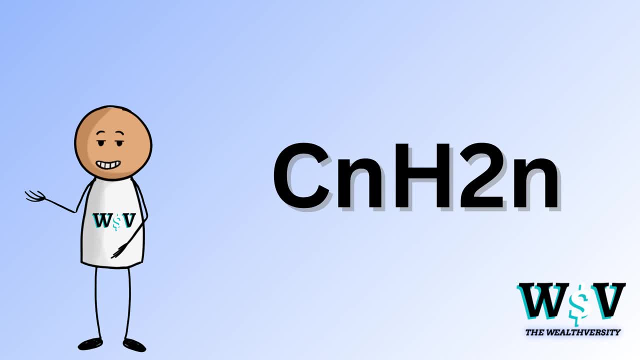 This means that you will have double the number of hydrogens, or 2 hydrogens for each carbon. The reason you have less hydrogens and alkenes than alkenes is because there are more bonds and less hydrogens in comparison to alkanes. What about the general? 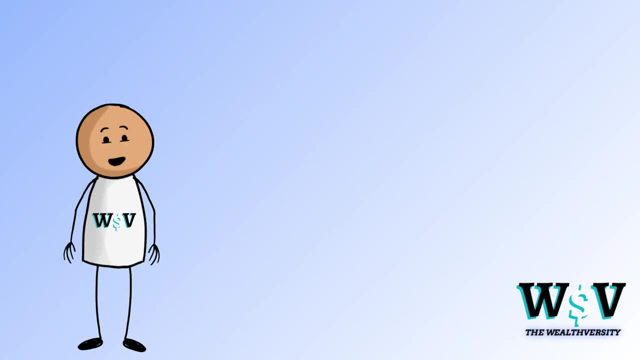 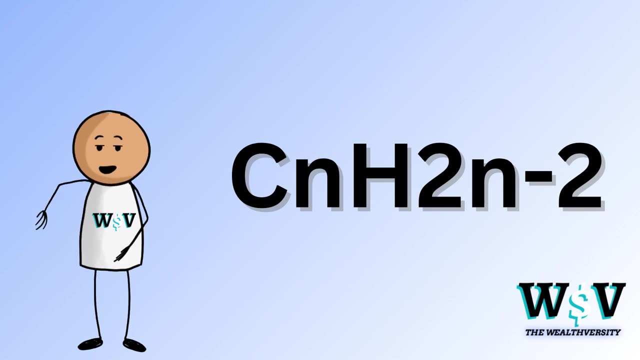 formula for alkynes. The general formula for alkynes is CnH2n-2.. This means that for every carbon you will have double the amount of hydrogens minus 2.. The more bonds you have in a carbon, the less the hydrogens. Let's see an example. So here we have ethane, ethene and 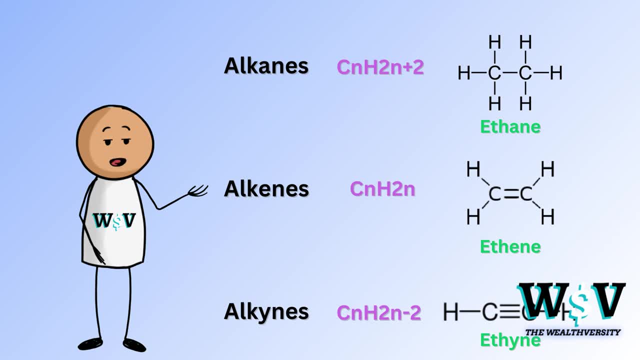 ethene. Ethane has a single bond between the two carbons and three hydrogens bonded to each carbon. Ethane has a double bond between the carbons and two hydrogens bonded to each carbon. Ethane has a triple bond between the carbons and a single hydrogen for each carbon. 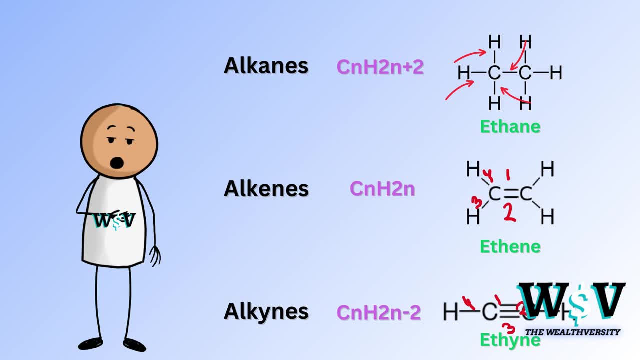 Notice how, in all three organic compounds, the carbons all have a total of four bonds. The only difference is: the more bonds between the carbons, the less bonds there are to hydrogens. Now how do we name alkenes and alkynes? Notice how an alkene ends in ene and alkyne with ein. 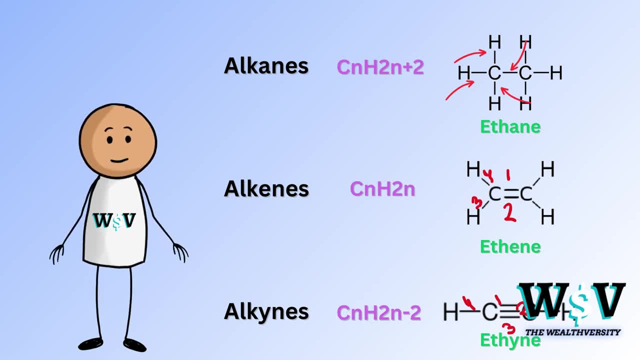 That is exactly how their organic compounds will end with. Everything else is pre-organic, Pretty similar to alkene naming. Let's look at a few examples, starting with an alkene. So we have this simple alkene First of all, just like all organic compounds. 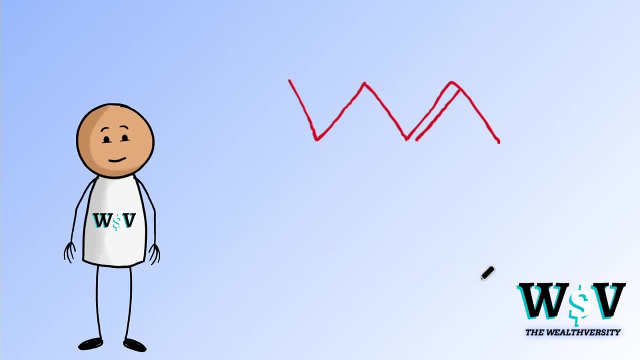 we look for the longest carbon chain, also known as the main chain, Since this is a straight carbon chain with no branches. the whole thing is the main chain. Now we see a double bond that is represented by two lines. For us to start numbering, the double bond has to be at the lowest position number. 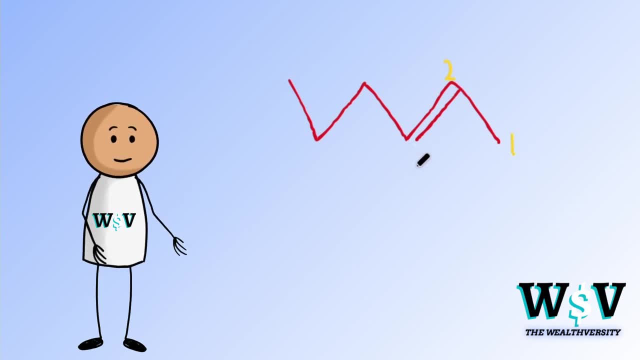 so we will start from the left, So 1,, 2,, 3,, 4,, 5, and 6.. So the parent chain is hexane. Now with the double bond, that is at carbon number 2, the end changes. First we remove the ene ending, then we add a hyphen. 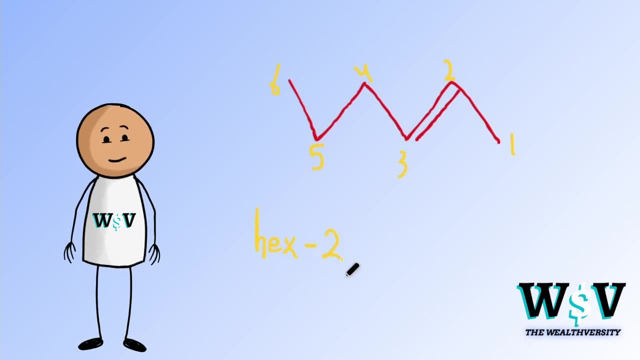 then we write the position number where the carbon happens, so 2, then hyphen, then, since it's a double bond, we write ene, So this compound is called hex-2-ene. Let's look at another example, a harder one. Wow, now we have three double bonds in a single compound. 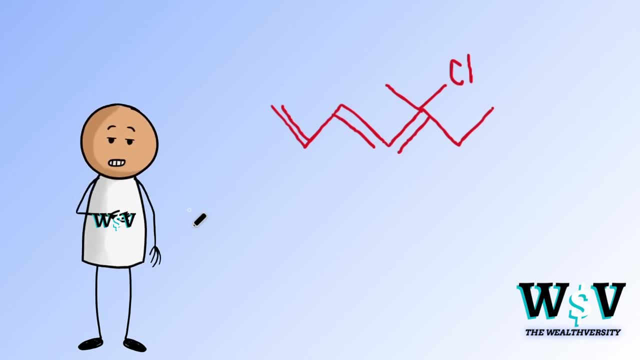 So how do we name this? Let's start by looking for the longest carbon chain possible. If we take this chain right here, we have 1,, 2,, 3,, 4,, 5, and 6 carbons. Let's try taking this chain. We have 1,, 2,, 3,, 4,, 5,, 6, and 7 carbons. 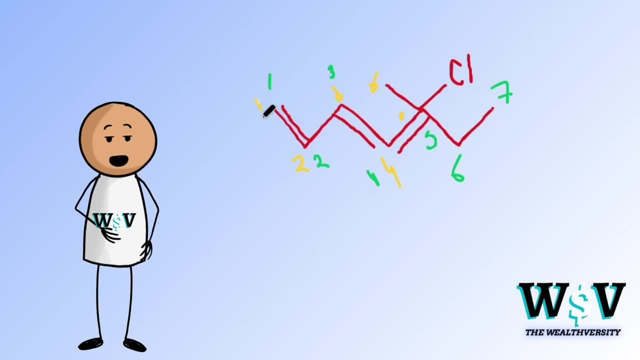 So this is the longest possible carbon chain. Now which way do we number it? We have a chloride branch, a methyl branch and three double bonds. so much going on. Double bonds will always take priority, So what you will have to do is number the chain in a way where the double bonds will have the lowest possible position number. 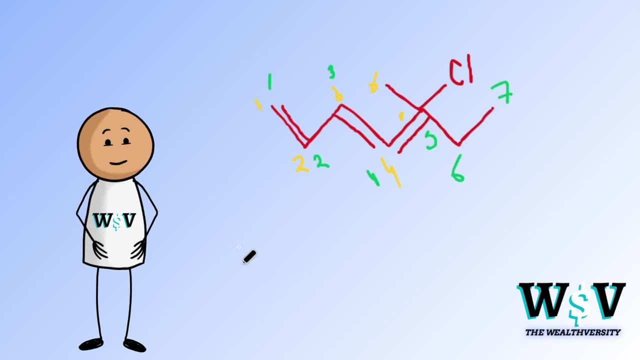 For the left side, the double bond positions are at 1,, 3, and 5.. For the right side, the double bond positions are at 2,, 4, and 6.. So obviously, numbering from the left side gives us the lowest possible number positions for the double bond. 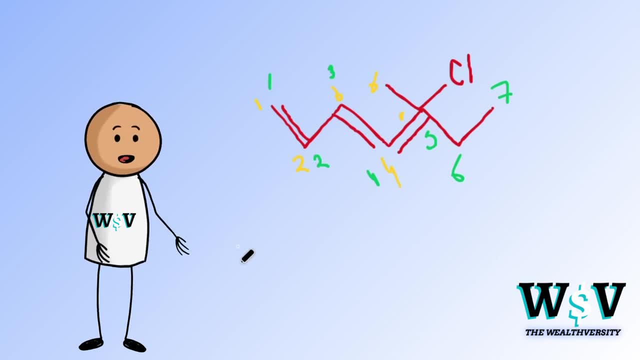 Now to number it. we start with the branches alphabetically, so the chloride comes before the methyl. The chloride is positioned at carbon number 5.. So we write 5-chloro, then the methyl is also positioned at carbon number 5.. 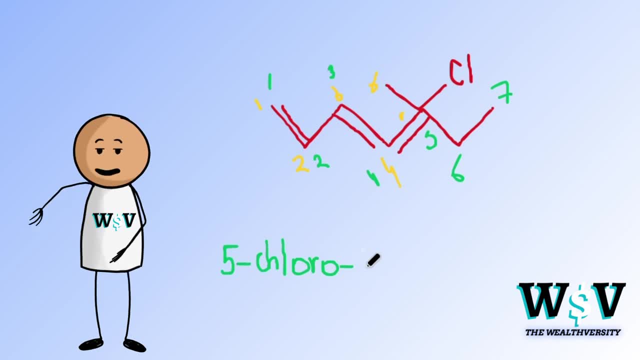 So we add a hyphen 5,, then hyphen methyl. Since we have 7 carbons, the parent name starts with hept, So we write hept, then we write 1,, 3,, 5,, since these are where the double bonds are, then hyphen trine. 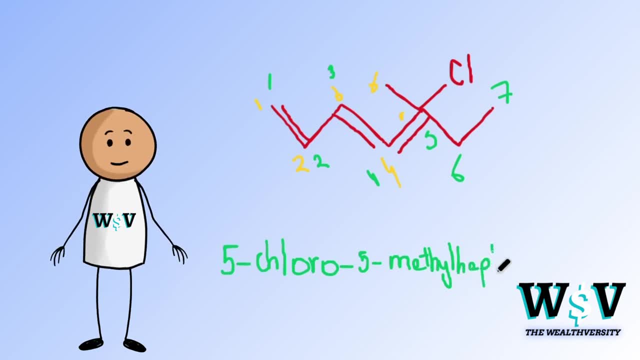 Since there are three double bonds, you have to add the trine. There is one more thing that we have to add: Since we have more than a single double bond, we have to add an extra a after hept, Just so the pronunciation makes sense. 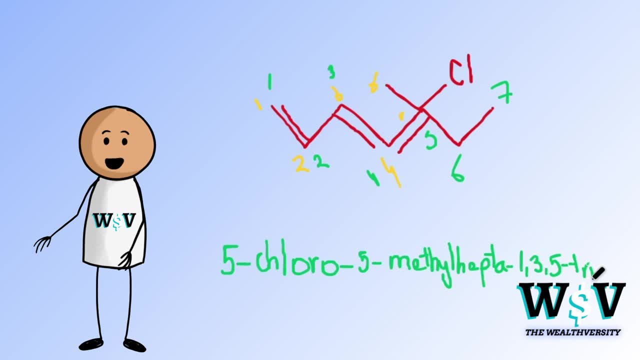 So this compound is called 5-chloro 5-methylhepta 1,, 3, 5-trine. It may seem complex, but once you practice it you will get the hang of it. Now let's move on to naming alkynes. 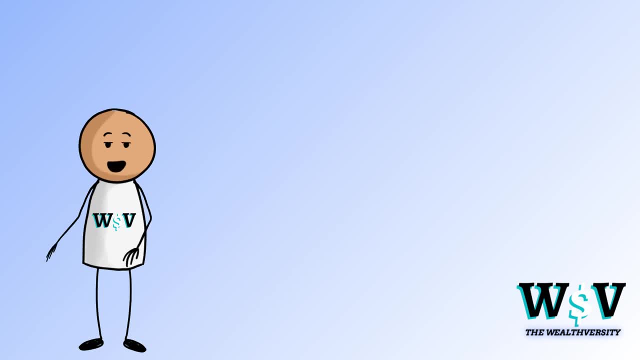 Naming alkynes is super similar to naming alkenes. They follow the same rules. The only difference is that alkynes end with ein. Let's try an example. So we have this nice and simple alkyne that has a triple bond and a fluorine. 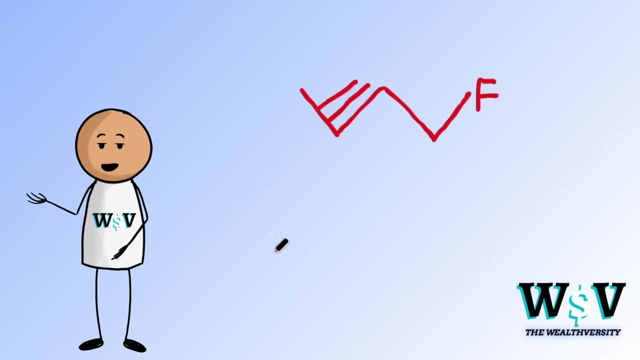 Just like alkenes, You must number so that the triple bond is at the lowest position number, since it has more priority than fluorine. This is a simple example and obviously naming from the left will give you the lowest position number for the triple bond. 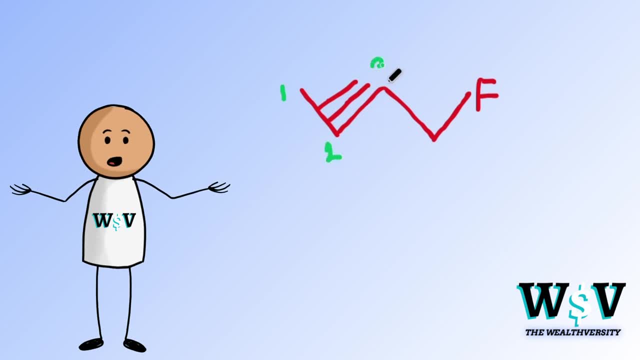 So we number it as 1,, 2,, 3, and 4.. The fluorine doesn't count because it's not a carbon. It's attached to carbon number 4.. Since fluorine is the only branch, we will start with it. 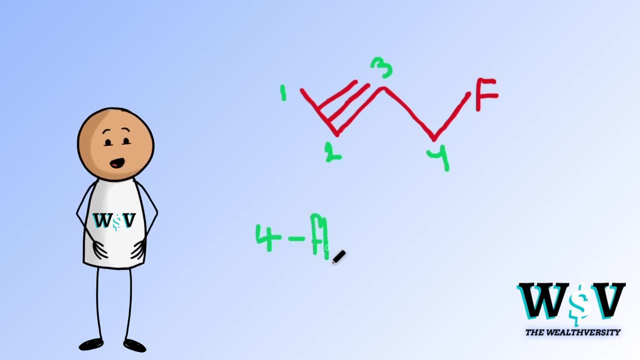 So we write 4-fluoro, then the parent chain is by it And there is only one triple bond. So we don't add an A. The triple bond is at carbon number 2.. So our compound name is 4-fluorobut-2.. 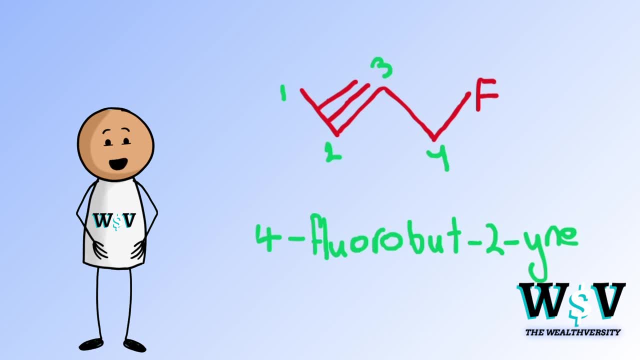 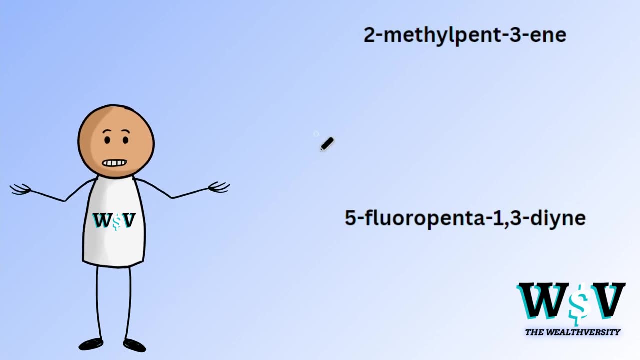 Very easy and simple And very similar to alkynes. What about drawing alkynes and alkynes? Take a look at these two names: One of them is an alkene and the other is an alkyne. Let's start with the alkene. 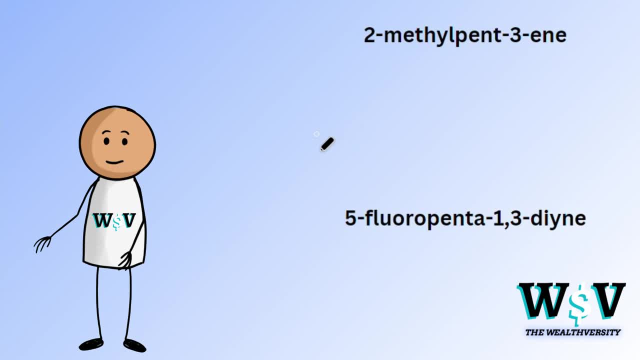 2-methylpent 3-ene is the name of the alkene. We can see that the parent chain is pent, So we have 5 carbons. So let's start by drawing 5 zigzag lines. You can also draw it using structural and condensed structure diagrams. 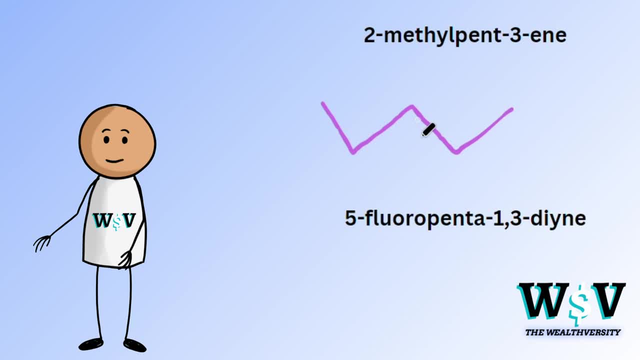 Next, we see that there is one double bond at carbon number 3, which is in the middle. So no matter what side you start on, carbon number 3 is in the middle And that's where we will add another line to represent a double bond. 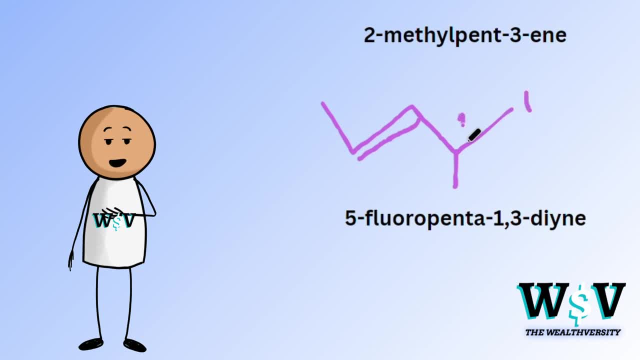 Lastly, we have a methyl group at carbon 2.. So you can either draw it here or on the other second carbon, Depending on which side you want to start. both are correct. Next, we have 5-fluoropenta 1, 3-dyne. 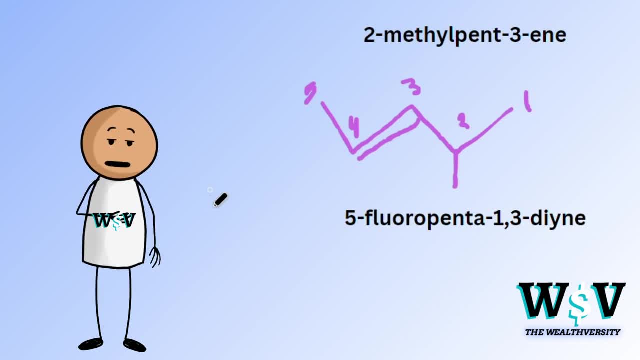 and alkyne. So, first thing, we can see that the parent chain is pentane, meaning there are 5 carbons. So we will draw 5 carbons. We will do a structural diagram this time. Next, we see that at carbon number 1 and 3 both have a triple bond. 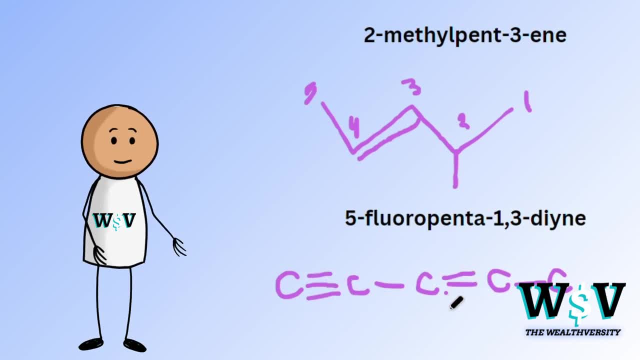 So we draw triple bonds at both carbons. Lastly, we see that there is also a fluorine at carbon number 5. So we will add another bond with fluorine to carbon number 5, represented For the rest of the carbons that have less than 4 bonds. 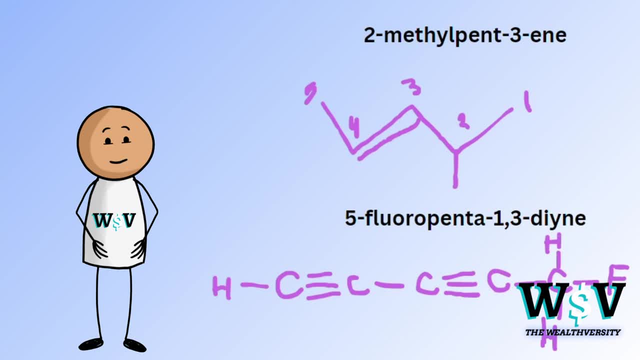 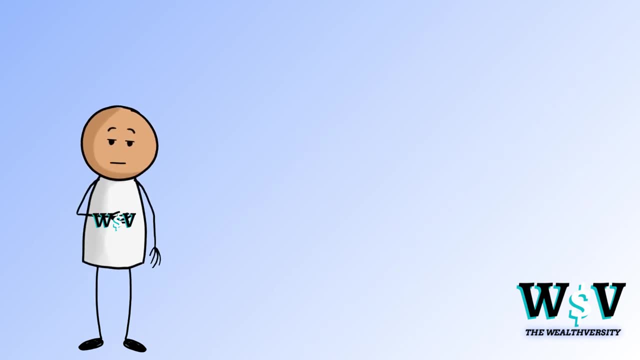 fill them with hydrogens until they have 4 bonds, And that's it Nice and easy. The more you practice, the easier it gets. That's it for alkene and alkyne naming and drawing. We hope you all enjoyed this video and learned something.